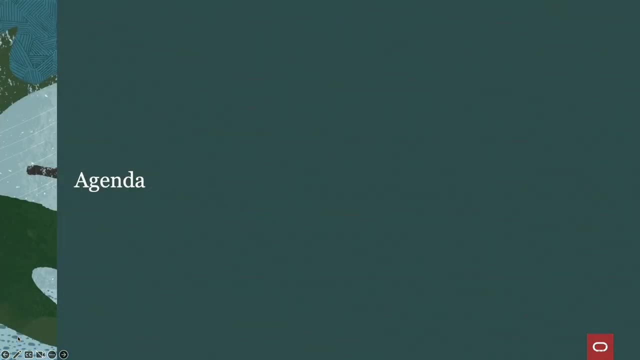 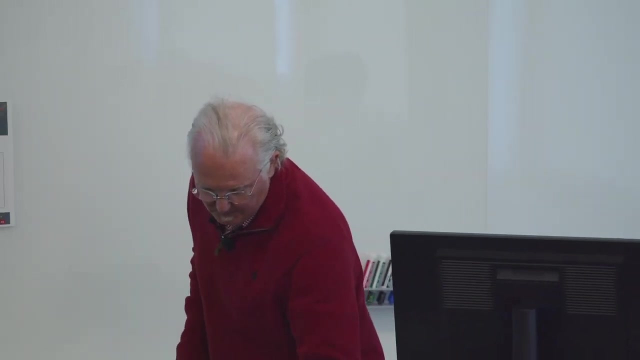 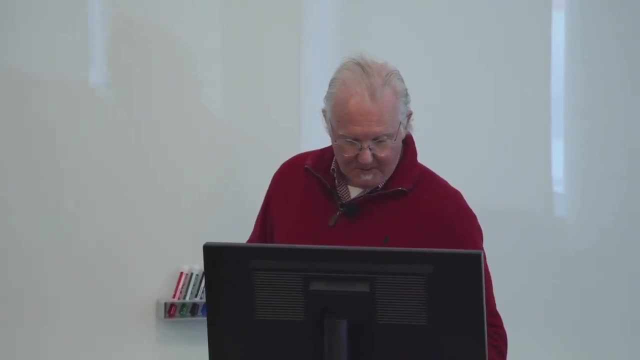 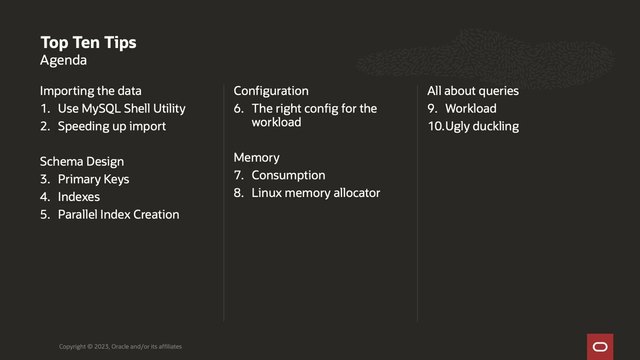 we're going to find out because it's got a lot of tips. There we go. I'm going to talk about a few things. I'm going to talk about how you can get data in or out of MySQL faster and into MySQL faster, and why you shouldn't use some of our older tools. so some new stuff. 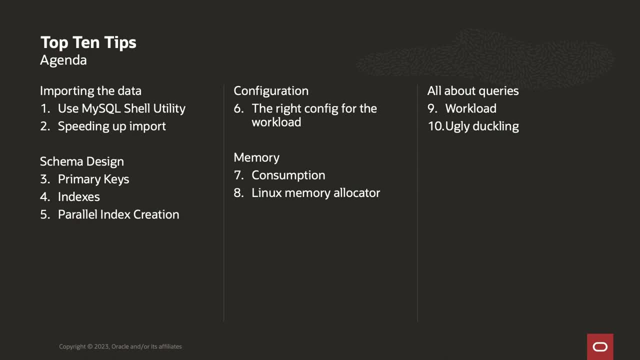 we have. I'm going to talk about some schema design things to think about and how to discover whether or not you have issues. so how to find it, how to fix it. We're going to talk about configuration, so how do you figure out what the size of your workloads are? so, 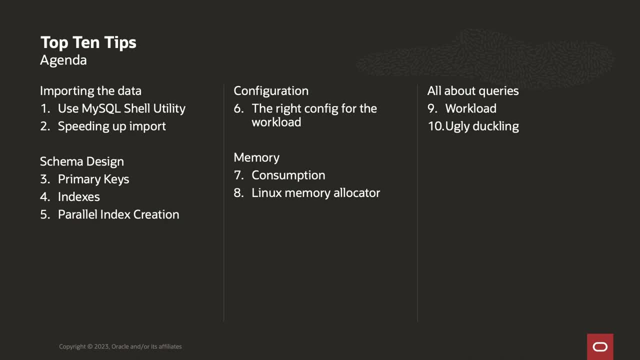 that you know how to set how much memory and things like that. Again, memory consumption: we're going to talk about that. We're going to talk about an alternative Linux memory allocator you can use that will greatly improve your performance and reduce the amount of memory used as we run on Linux. We'll talk. 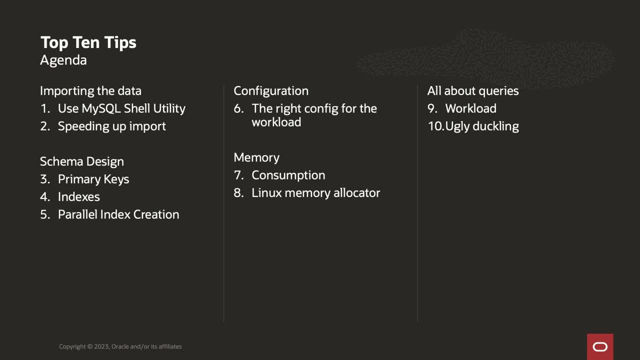 about looking at your workload, determining how many reads, how many writes, what's my ratio, how should I set up? and then the ugly duckling, as Le Fred named it, and that's what's your worst right. Let's go fix that. 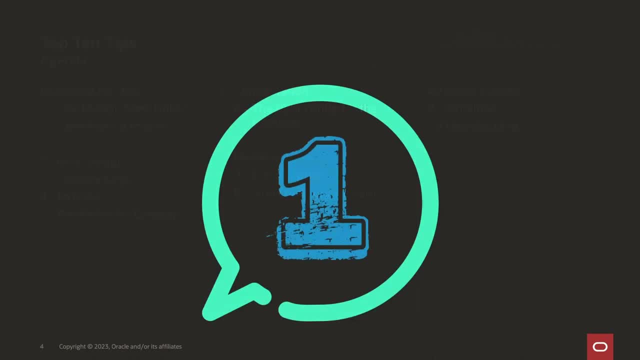 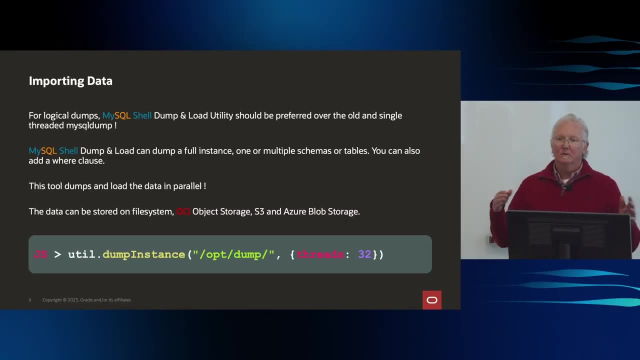 And then rinse and repeat. So let's see if I can get through this. So, number one: importing at the speed of light. And so MySQL. we had the MySQL dump. It's been around a long time. It's single-threaded, It's not that fast. We have MySQL Shell. now It's got an export. 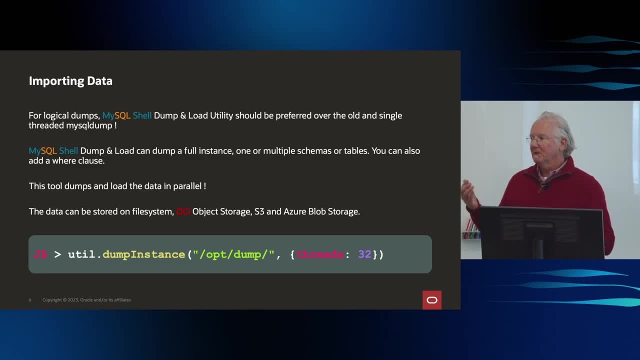 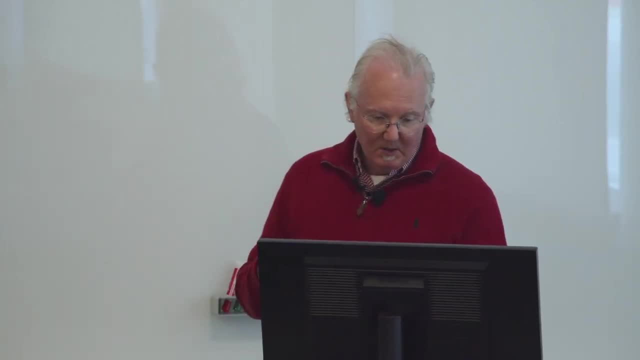 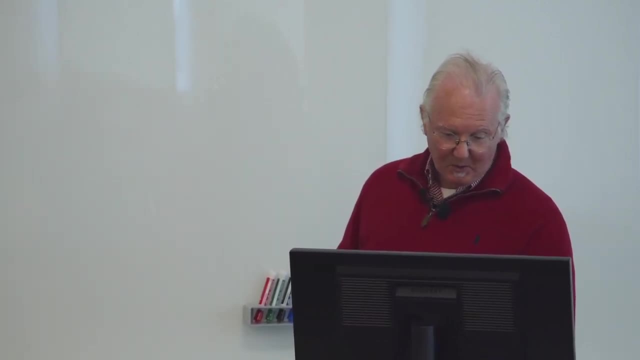 and import utility. You can dump an instance, a table, a schema and you can determine how many threads it uses. Export faster And you can do that to object: storage of various flavors. I'm going to go fast, So that's what that looks like, But then when I import the data, I can conversely. 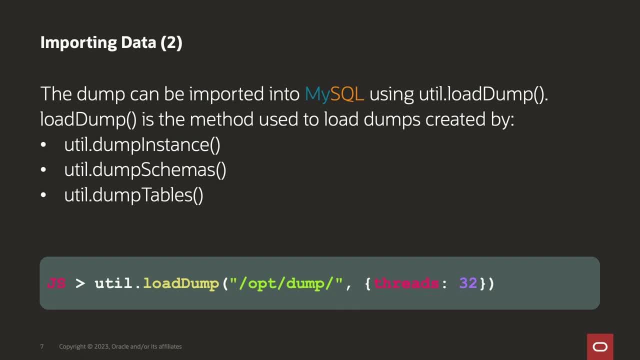 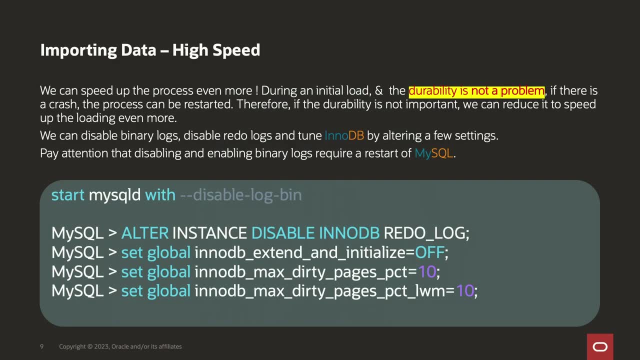 also determine how many threads I'm going to use to import it, right? So bring it in faster with more threads Then sort of related to this, right? So if I'm setting up a new database, I'm importing a bunch of data. 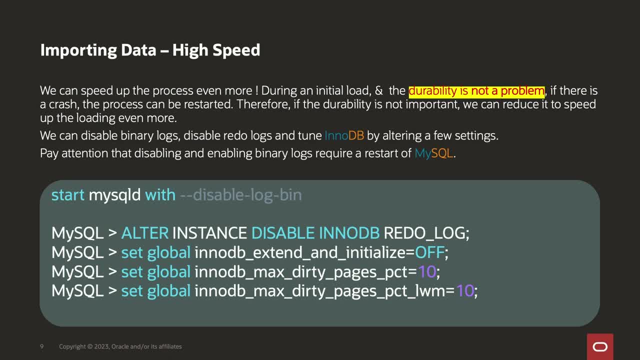 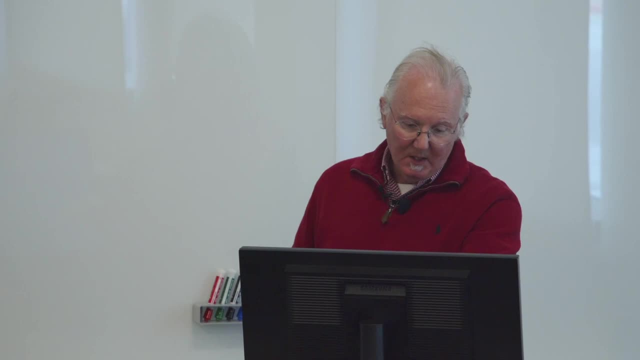 I don't care if I have crash recovery and things like that, Then I can go in. I can disable a redo log. I can turn off the bin log. Now I'm not going to do all that IO for that, And so when I do my import it's going to go in a lot faster, So I can go in. 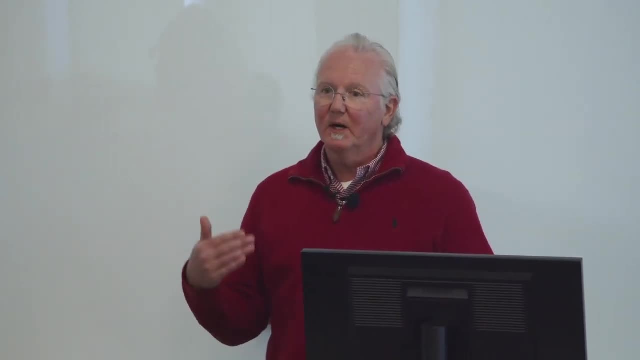 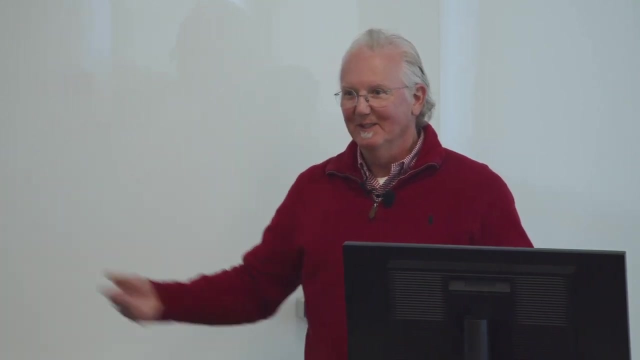 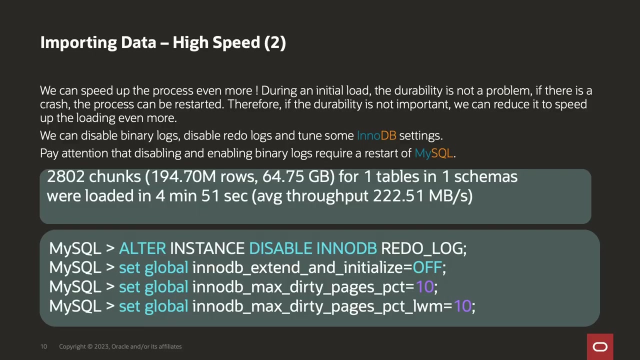 change those settings And then, FYI, after I do that, I'm going to have to change them back and restart the server so that you obviously do want to have a redo undo and a bin log right, And so we can speed it up a great deal. And here right he's showing that he got 222. 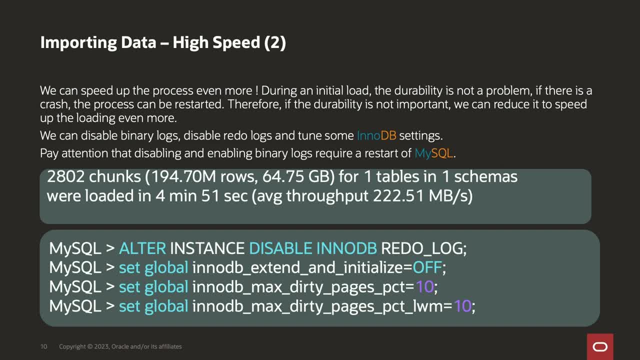 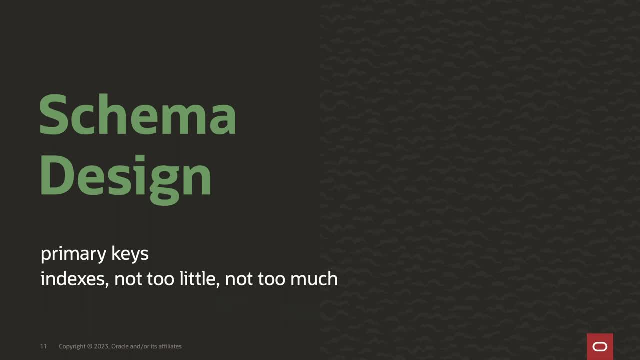 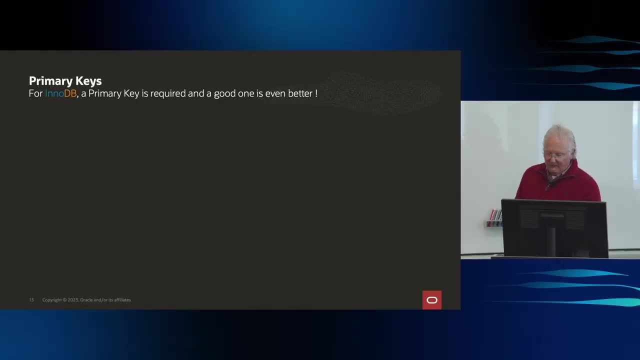 megabytes per second, which probably on the disk system he had, is about as fast as that thing could go right, So that you'll max things out a great deal, All right, Number three: the primary key. All right, So we have to, we want to have. 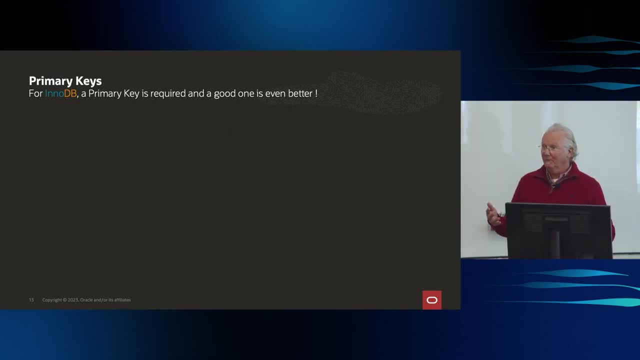 a good primary key, And there are such things as no primary keys and bad primary keys. So let's, let's think through this. So you know, obviously we store data in a table space And when we have a primary key, it's on a clustered index, right? That's the primary key, But we also have secondary. 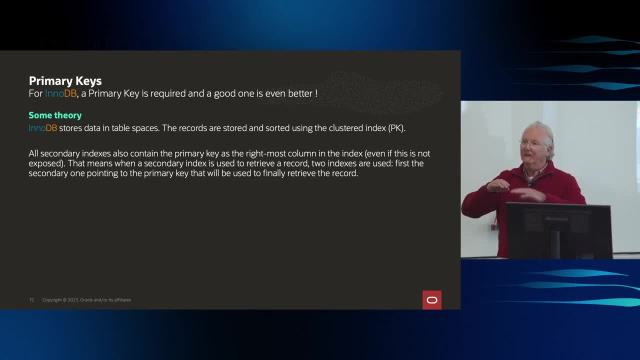 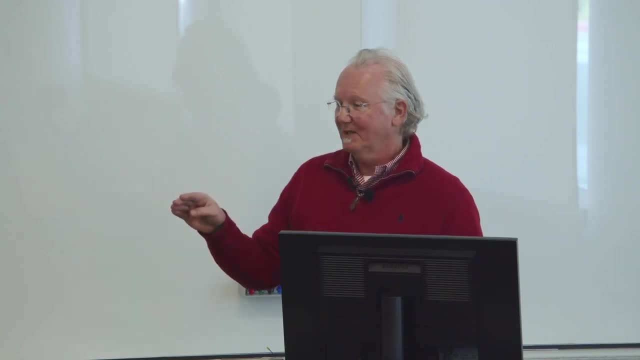 keys right And those secondary keys have to refer to the primary key to find the row that you looked up if you searched a secondary key right. So the primary key is always going to be used right, Unless you're doing a full load. 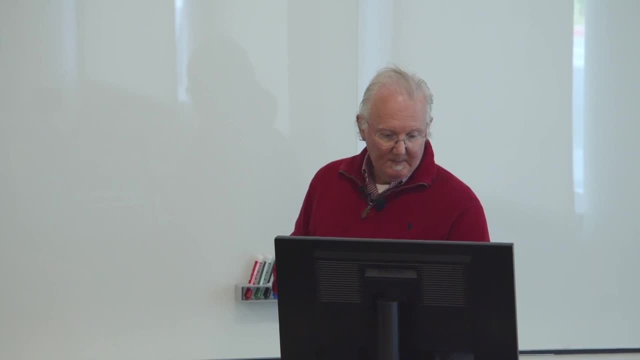 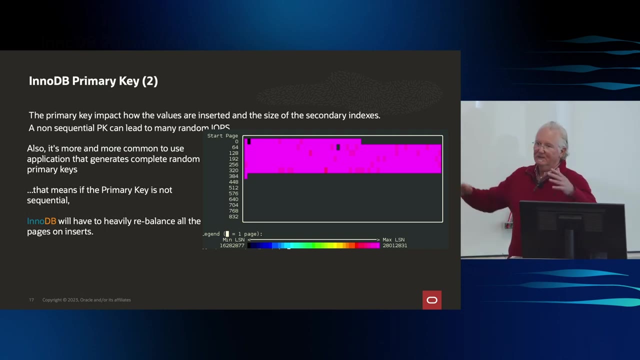 A full table scan or something like that. So if we have a non-sequential primary key, the problem is that it's got to. you've got to reorder your tree right, And so when you reorder your tree, all this pink is activity right And that's bad right, And so we don't. 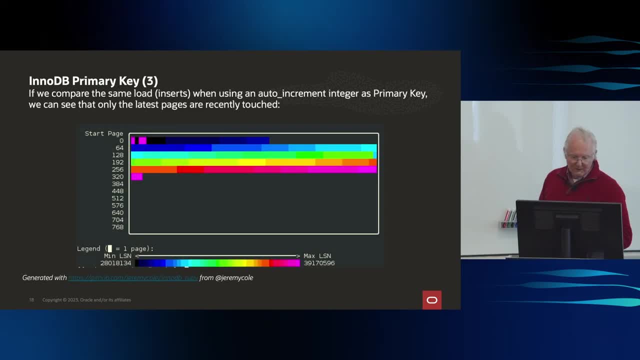 really want to do that. What we want to do is we want to have a monotonically increasing positive integer, right. And when we have that and we're adding new rows with these auto-incremented things, right, then we're not going to be rebalancing things so much. 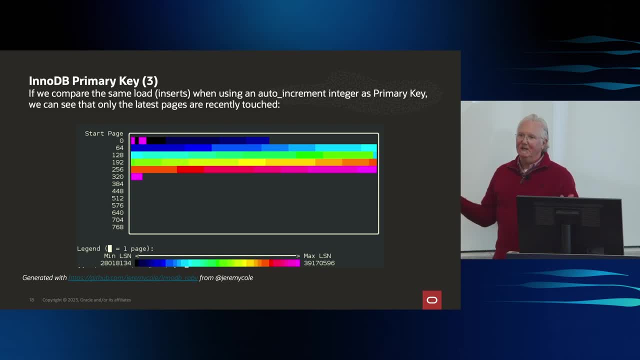 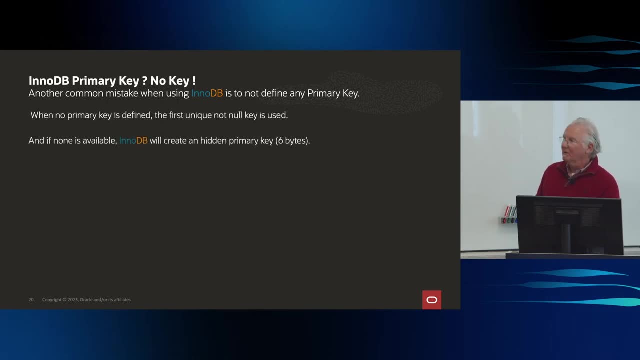 right. So here we got a lot less pink. So that means less pink means less performance, less pages are changed. And another problem is that if you don't define a primary key, we have to have a primary key right. So we're going to create a hidden one right. 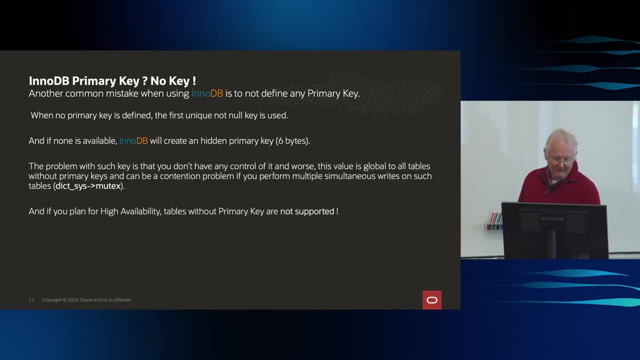 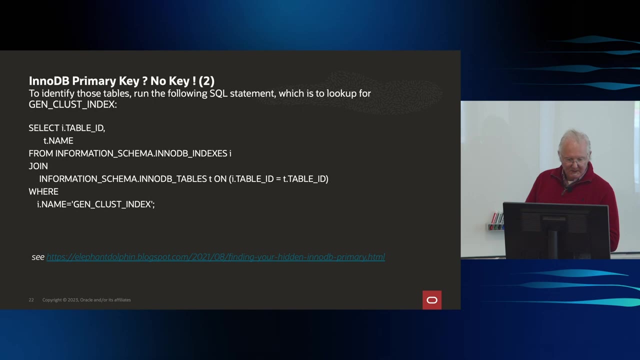 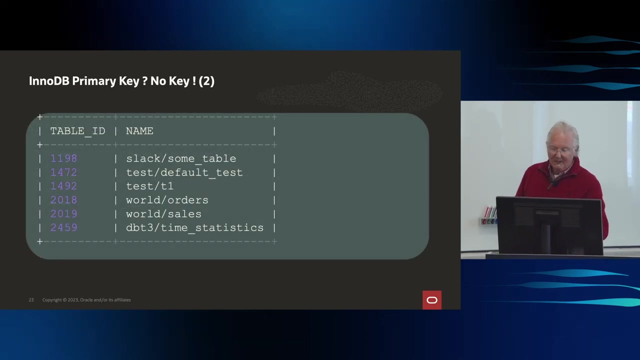 And those are six bytes long. So it's really you don't have control over this thing, right? And so really you should define a primary key And even more than that, let's see. So how do we determine those tables? Well, we run this query and we can determine, okay. 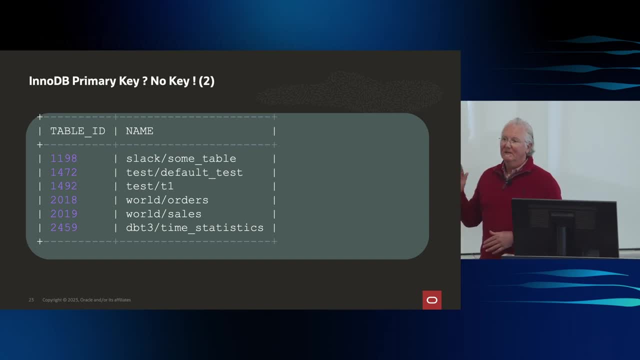 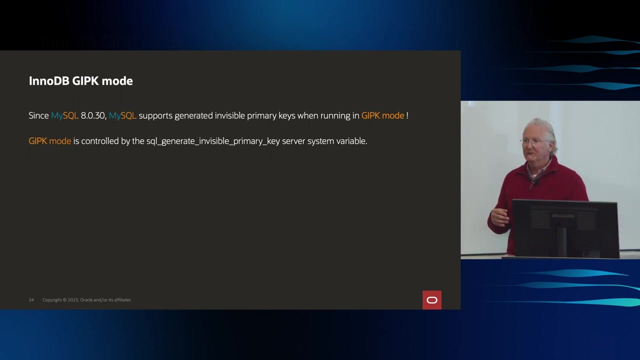 these are the tables that I haven't defined a primary key. That's probably not a bad idea. Obviously there's a hidden one And that's a problem, All right. But now we have a new mode. It's called generated invisible keys, So sometimes 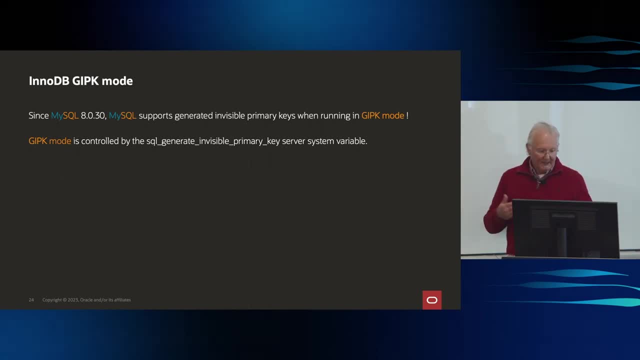 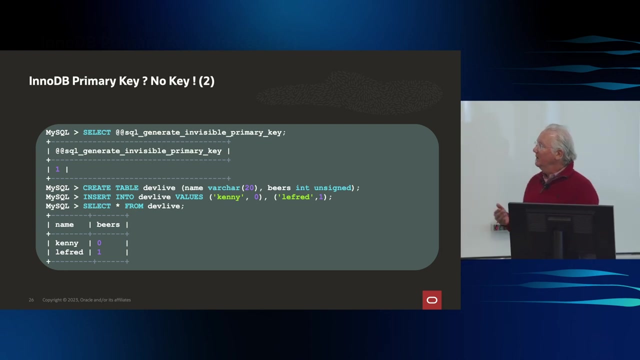 you don't have control over the schema and things like that, And so this will automatically generate keys for you And the primary key is just added to the table. And so in the case where it's on right and I create a table, say, I create a table like this, right? So 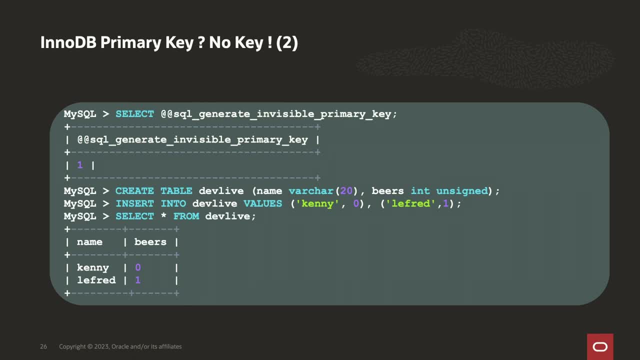 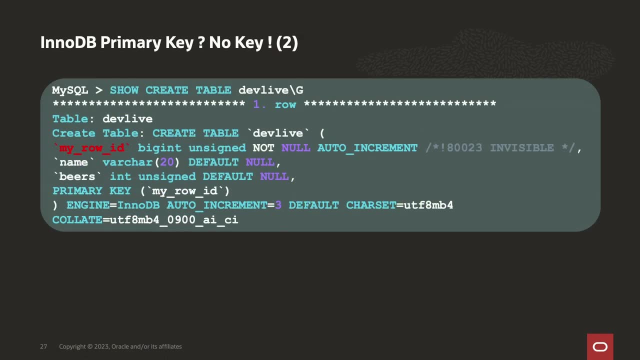 it just looks like there's name and beers there for Kenny and Le Fred, who love Belgian beer. But if I show the table right, I can see I have my row ID right. So this automatically generated this row ID for me, right, And it's an auto increment and it's a big unsigned And that. 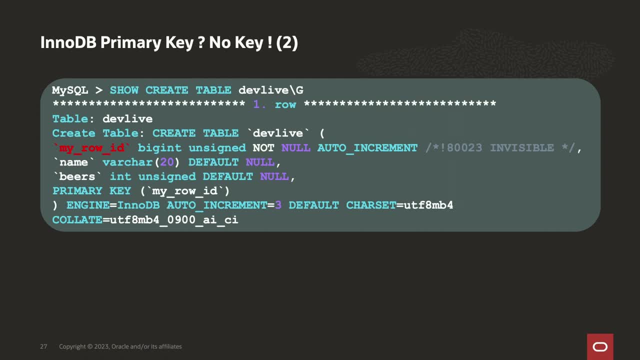 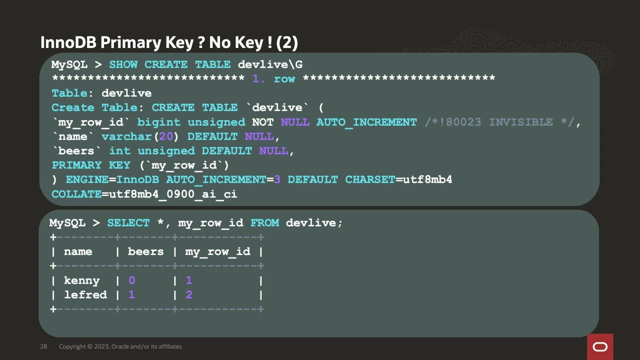 you know you have to. if you're doing HA, if you're doing DR right, you have to have a primary key right, So you're going to see that right there And so I can actually get that value right. So if I, if you, 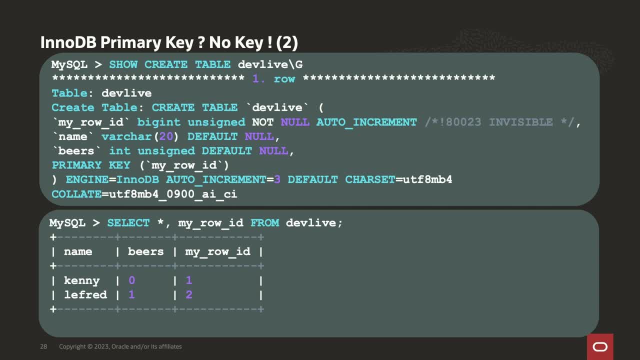 do a select star, you're not going to get it. But if I do a select star, comma and my row ID, you can get it And it's. it's really important to have a unique row ID for a lot of reasons, But like 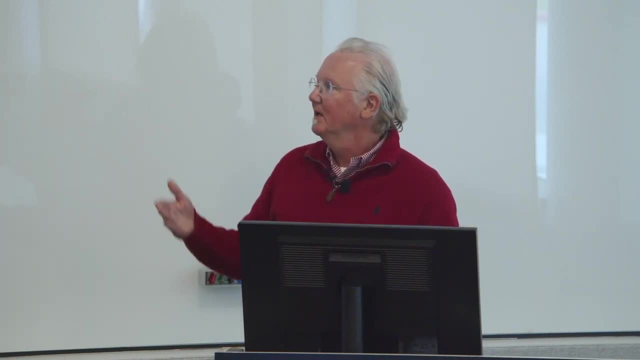 if you're trying to do data deduplication or things like that, right, you might need that row ID and you can use that to go In and determine. okay, I'm going to remove one of those rows. it's a duplicate or something like. 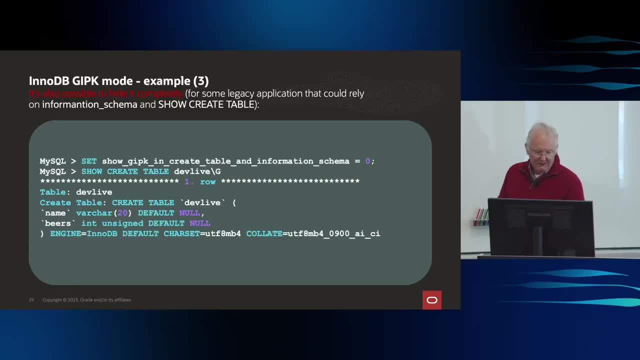 that It's also possible to hide this thing. So some tools out there read the data dictionary And if this shows up in the data dictionary, that and you're using some sort of a worm or something like that that could throw it off, Right, so you can hide it. 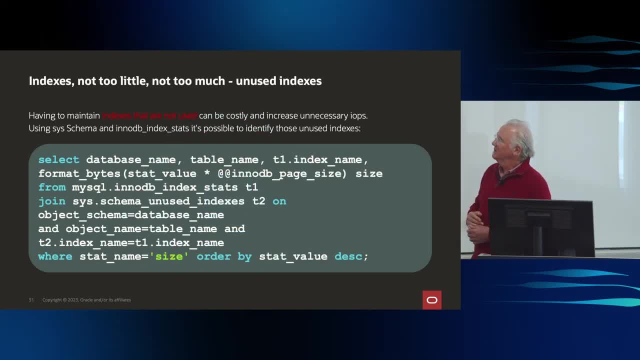 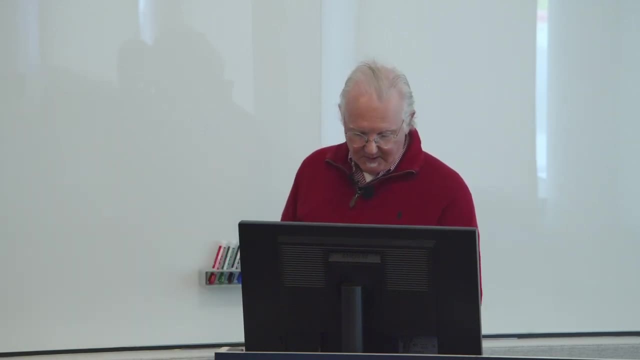 All right. tip number four: index is not too much on the not too little, not too much, Right. So you don't want to over index because an index is something you have to write and maintain and all that. But you definitely need. 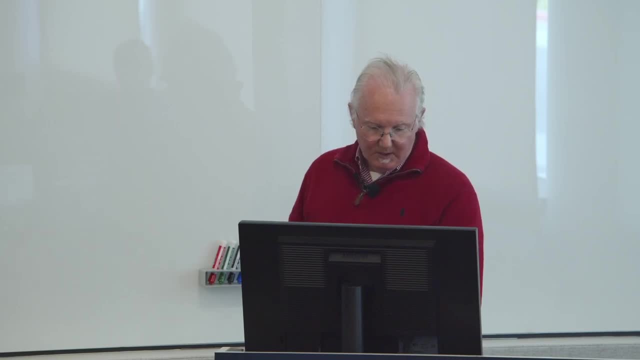 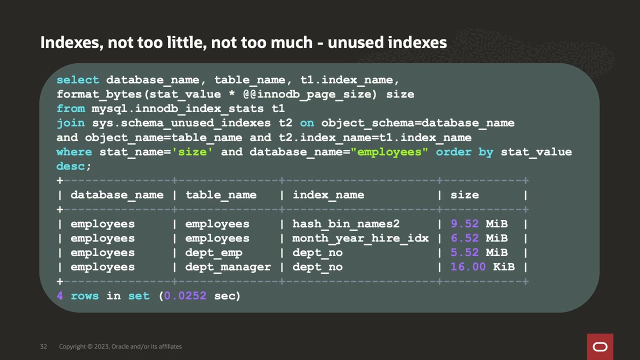 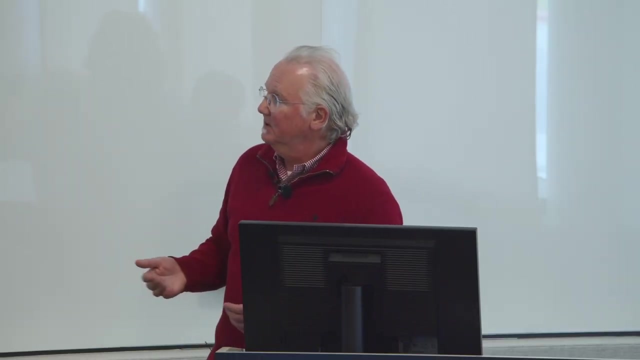 to have them, And so we can run this query And we can determine. let's see what. what hasn't been used. These are indexes that have never been used, So if they've not been used, just drop them right. 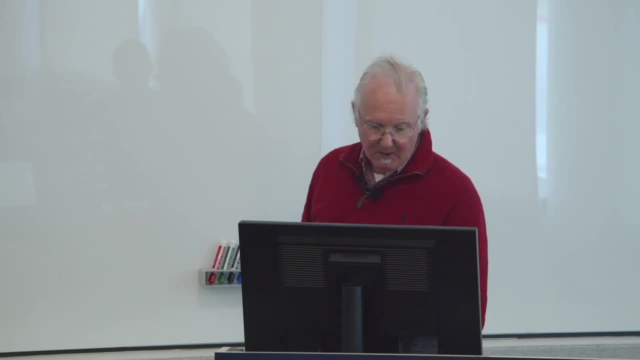 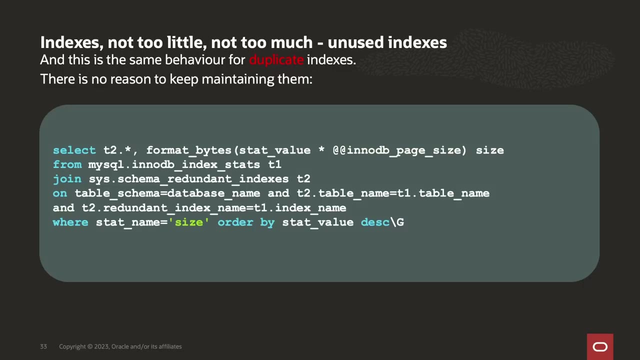 If no query is ever used in this thing, you don't need them, So get rid of them and drop those unused ones. But then the other issue that you almost see is sometimes people create duplicate indexes on the same column, right, You don't need that either. 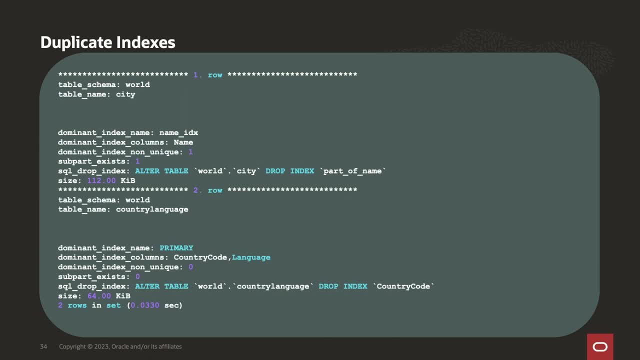 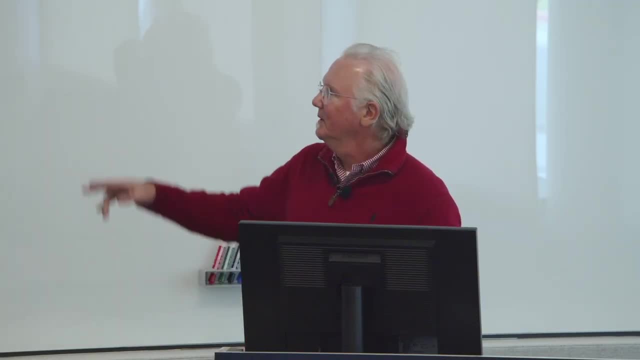 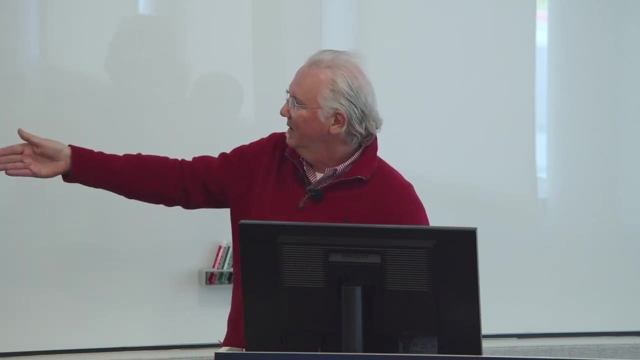 And so we can run that query that I had on the previous page and then it'll actually the way it's written. it'll spit out. okay, you need to drop alter table. drop these two indexes, because there's already an index on the world city and on the country language. 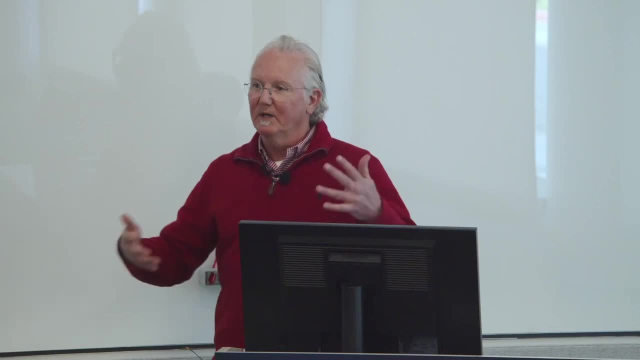 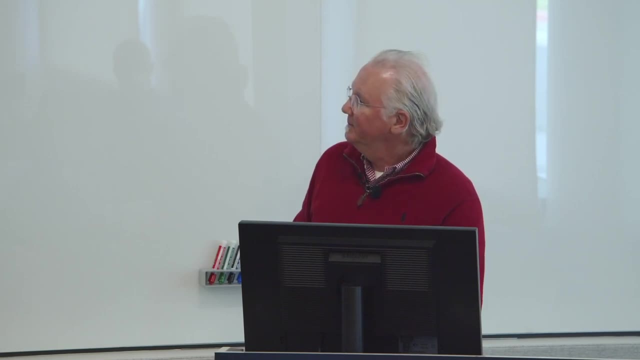 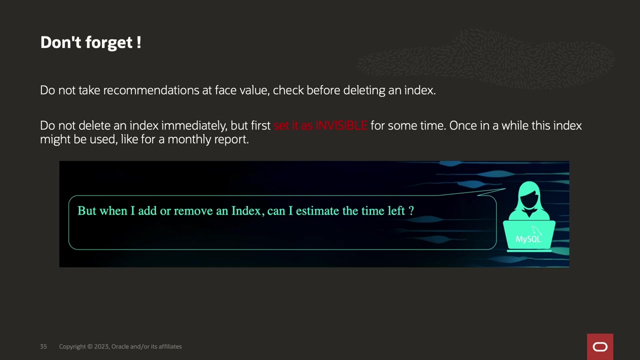 Right, there's two of them, Because we don't prevent you from creating two, and maybe there's some edge cases where you'd want to, but we tell you that, All right, don't forget. Oh, yes, so if you've got a really big table and you think that index isn't used, 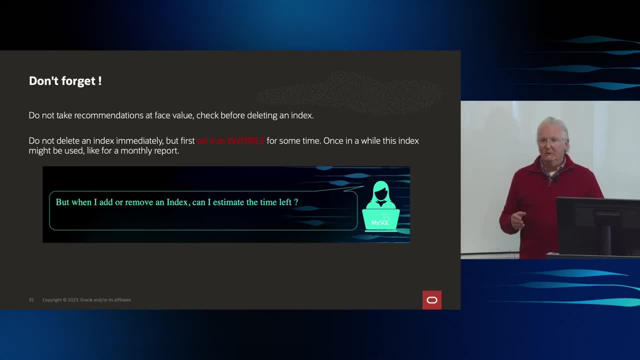 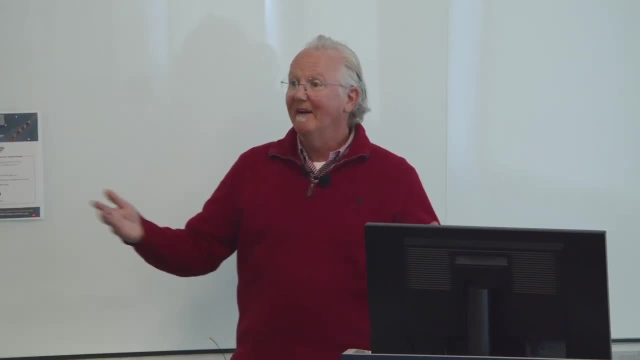 so maybe you don't want to drop it, Maybe you want to set it invisible and see what happens, right? So if you set it invisible, the optimizer is going to not think it's there, but it's still going to get maintained when you do insert. update deletes. 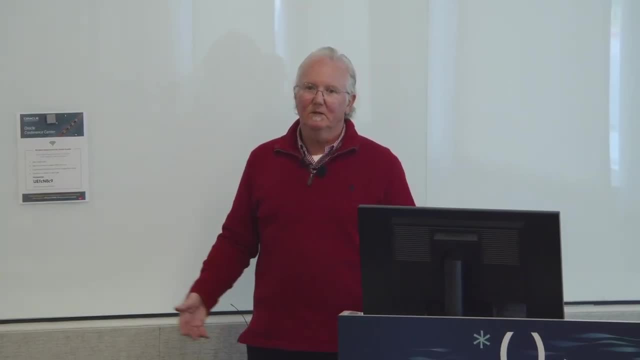 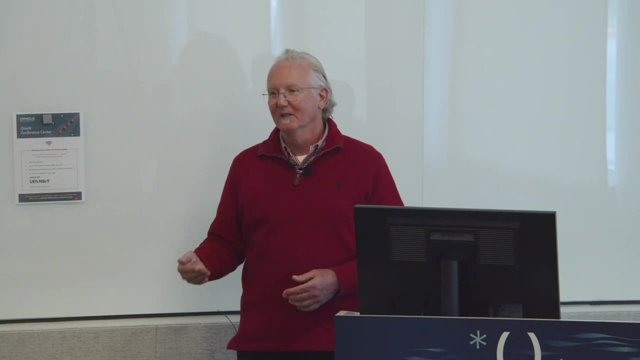 But then all of a sudden somebody goes: what You get? my, my Latency on this query. it's taken forever. And you're like, oh well, I dropped the index on it. So then you just set it invisible. but if nobody complains you drop the thing, right. 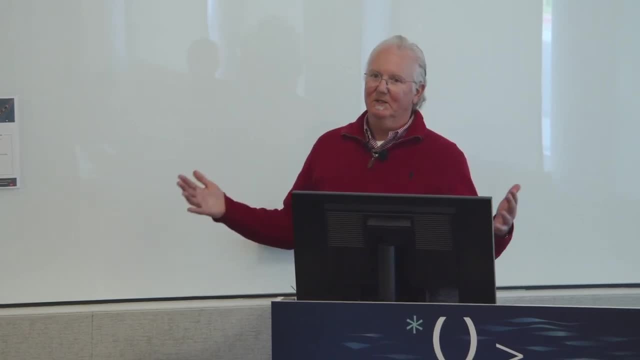 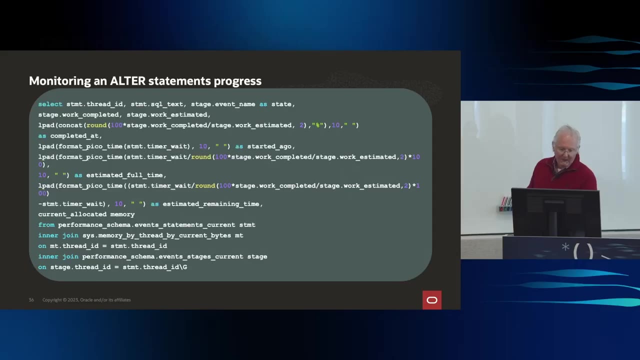 So you have an option there to not shoot yourself in the foot, because on billions of row tables, creating an index takes a while. It's a lot of effort. Also, when you go through and you do an alter statement or something like that. 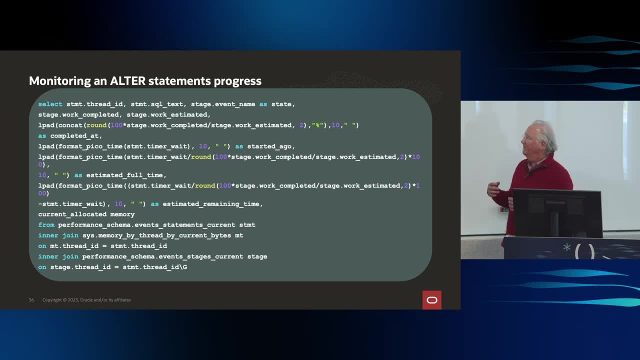 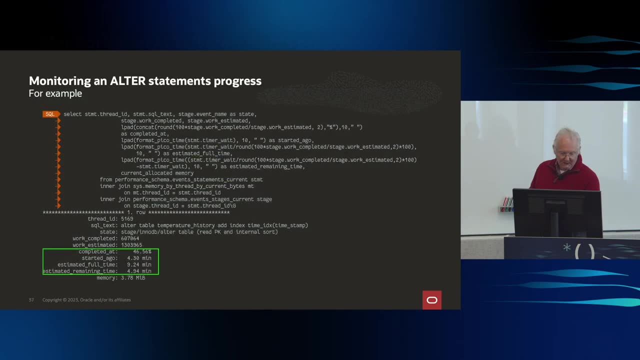 you can actually watch and see what's going on. So if you're altering it, If you're altering an index or something like that, you can run this statement and it'll actually tell you: okay, it's 46% done. You know we'll be done in another four or five minutes here. 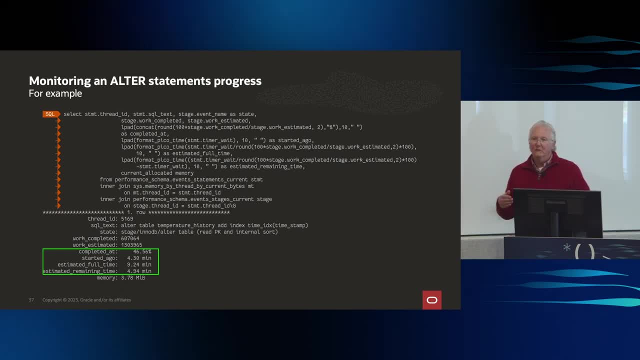 You know you can get there. So this ability to monitor alter statements is really a nice one, because there's nothing worth it. You know it's just sitting there running and you're like what's going on? This is going to. 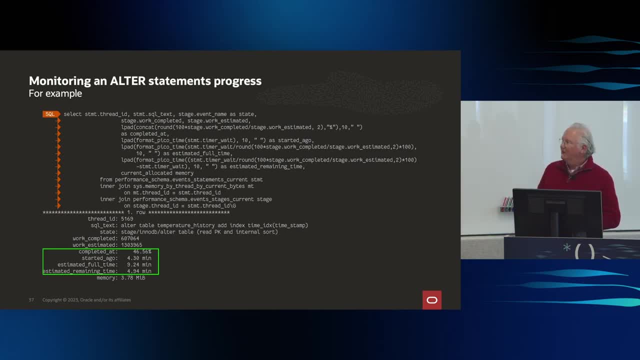 Is it making any progress? Right? You can't tell This way. you can tell. You can run this over and over, Watch it until it completes, and then you know you've got your job done. So also, we need to know, okay, what's missing, right? 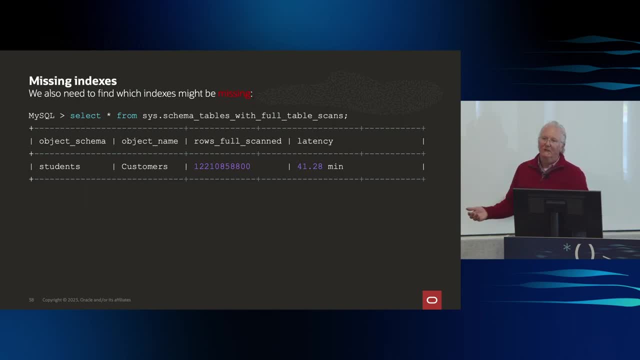 So we can look, for example, and see if there's a full table scan. there's not an index being used, And so we can easily select from this sys table right and we can find out what's missing. We can see that. 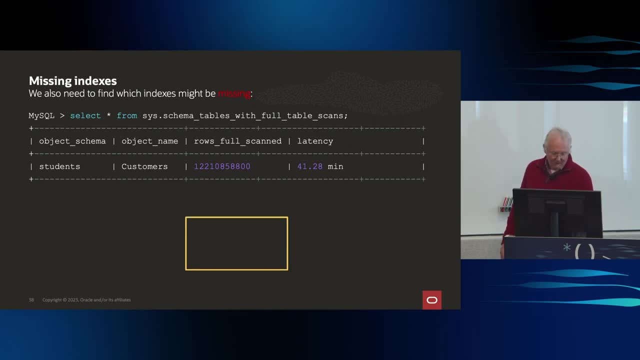 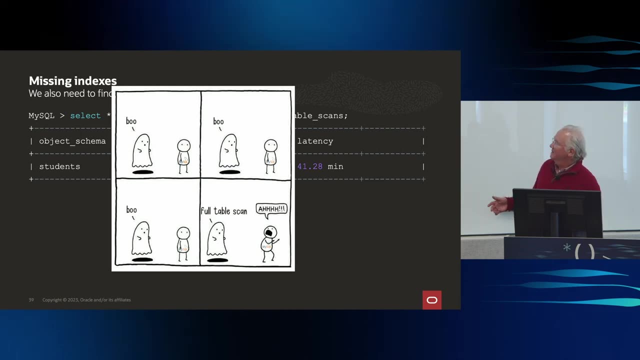 This 41-minute. Wow, that's a long query right. A lot of rows getting scanned. So if you're a DBA, right- and this is the LaFred humor, but you might be not scared by Boo, but a full table scan is terrifying. 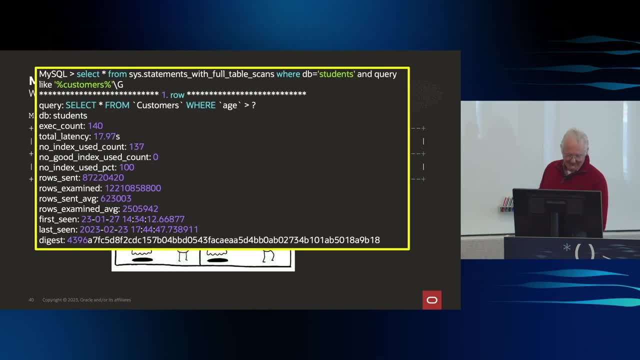 It's got a giant table. So we're going to look at this one and we're going to look at the find the query, And so it's going to be, you know, this whole table. that was doing the full table scan. 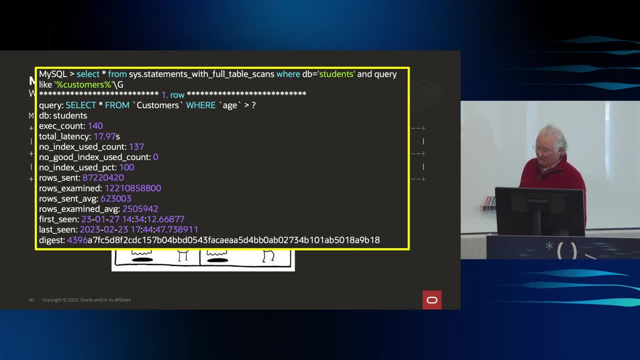 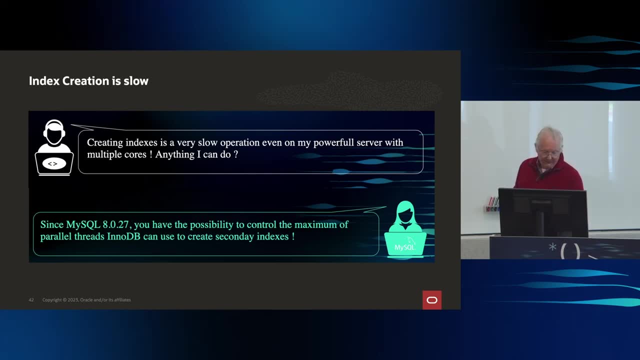 And we see it's select from students where age is greater than whatever right And its age is not indexed, And so now we know where our problem is. All right, So number five, So another thing you can do, going forward, right. 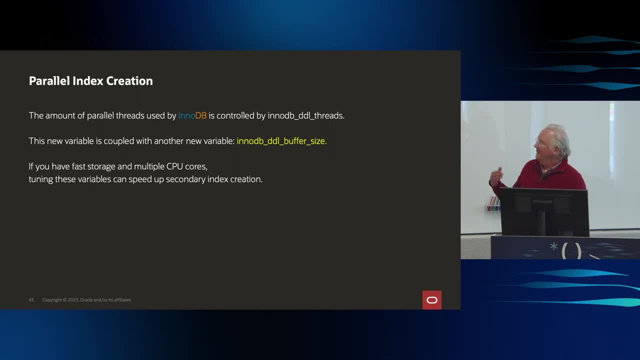 is, it takes a lot of power to create indexes. We can add buffer and we can add threads to this, And so, for example, this particular alter table took nine minutes- right, That's a long time. And that was done with four threads- whatever that is in buffer size- and four parallel re-threads- right. 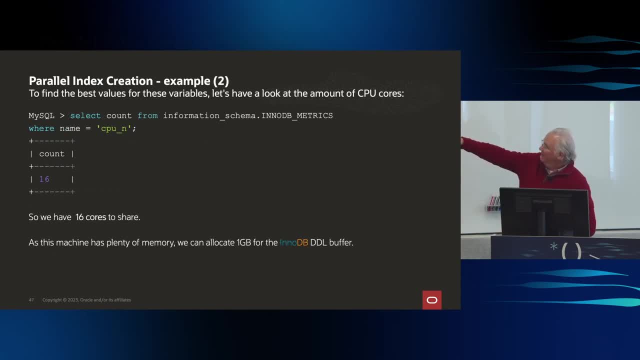 But if I go in and I look and I say, well, how many CPU cores do I have? Well, I've got 16.. Well, I can use more of that. So I'm going to set my DDL threads to eight. 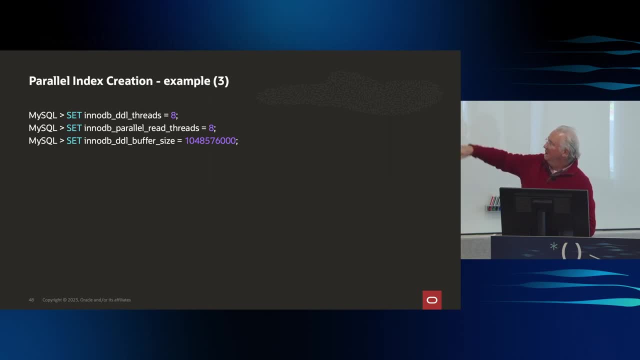 I'm going to set my re-threads to eight for the 16.. And I'm going to up my buffer size, because if I've got more threads, I need more buffer to do this. And so now I do it, and voila, I just did it in under three minutes versus nine minutes. 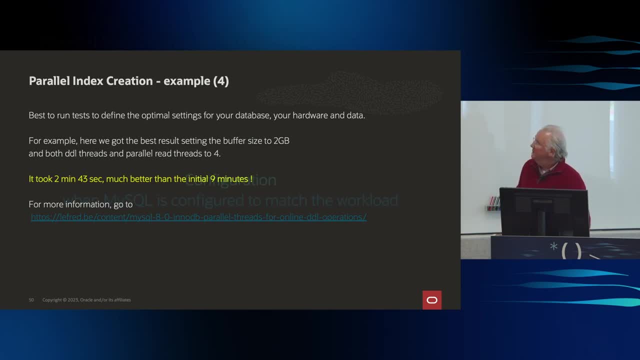 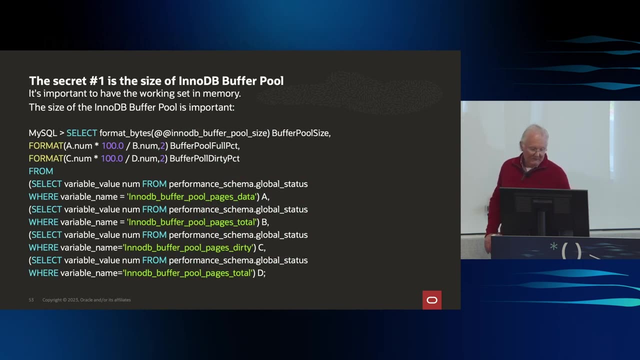 So I tripled my performance on that. All right, Let's see Number six: Buffer pool size. All right, So it's important to know sort of the size, how much of the buffer pool you're using, right? So if you run this query and again everybody will get these slides, then I can see my buffer pool size. 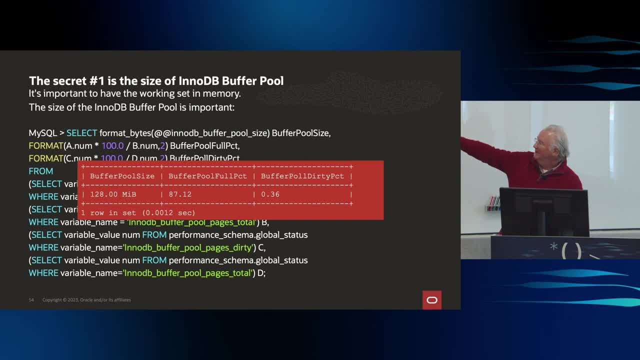 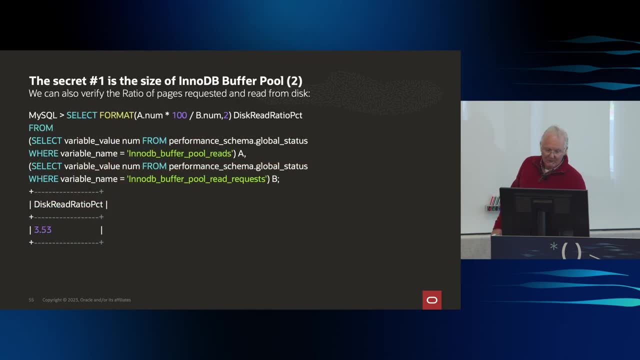 I can see how full it is And I can see if I've got many dirty pages in it, right, which I hardly have any in this example. So, and then I also may want to know: okay, how many reads to writes do I have as well? 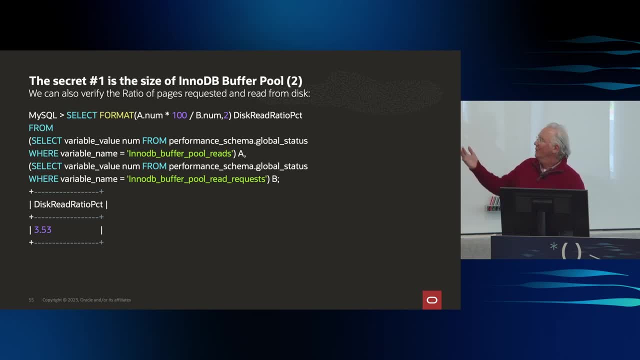 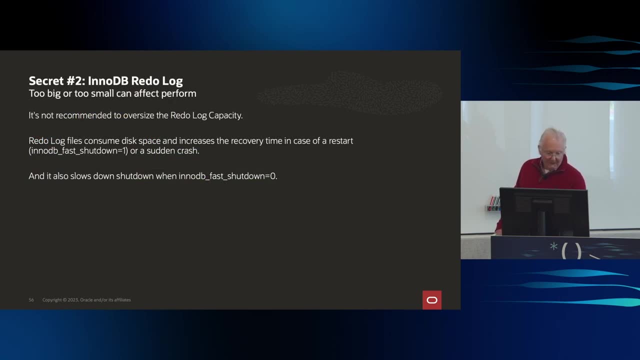 And obviously if I have a lot of reads, I want to make sure that these pages are hot there in the buffer pool. All right, So the redo log. So the next thing is: okay, how big should my redo log be right? 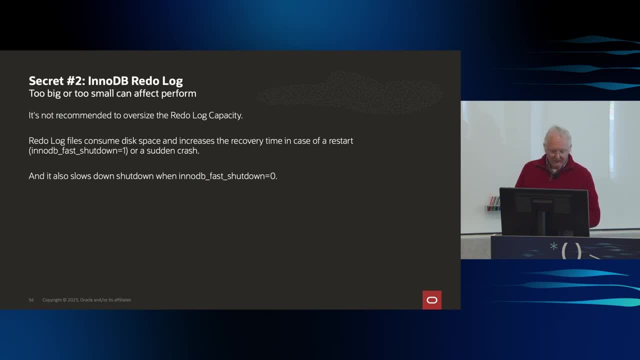 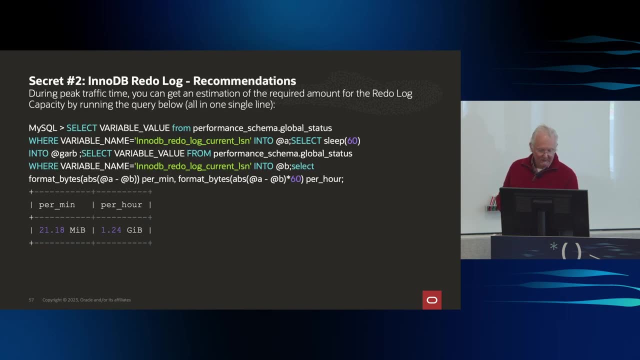 Well, if it's too big, it can affect performance And I can have issues on how quickly I can shut down or I can recover if it's too big. And so if you have a peak traffic time and you run this query right and this particular one will show me how much, how many megabytes, I'm using per minute and how many gigabytes, for example here that I'm using per hour, 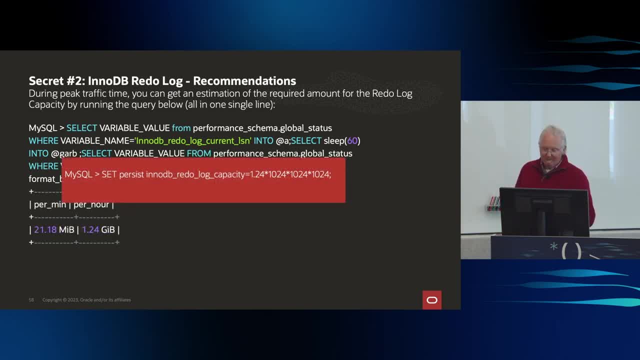 And so the recommendation Is that. you know you probably need about an hour's worth, And so I'm going to change my redo log capacity to that, And whether that's higher or lower, it's the right size, right, You don't? you just don't want it to be too big. 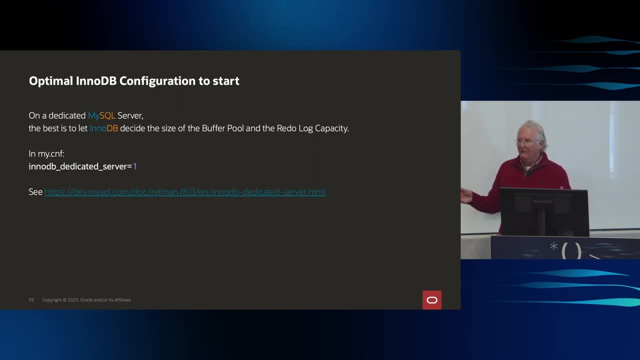 The other thing is that you know just by default. if you don't know some of these things, then let us set them right. So just say, hey, dedicated server, We'll look at what sort of resources you have on it. 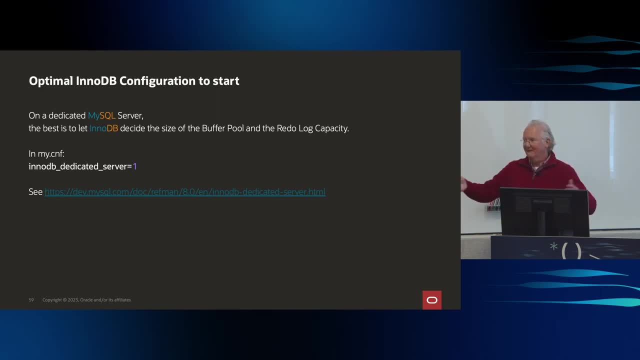 And we'll use everything. Now, you only want to do this on a server that's dedicated. That's why it's named that. Right, But we can pretty much beat anything probably you could come up with. if you don't, if you're not a super expert like Dave Stokes or somebody. 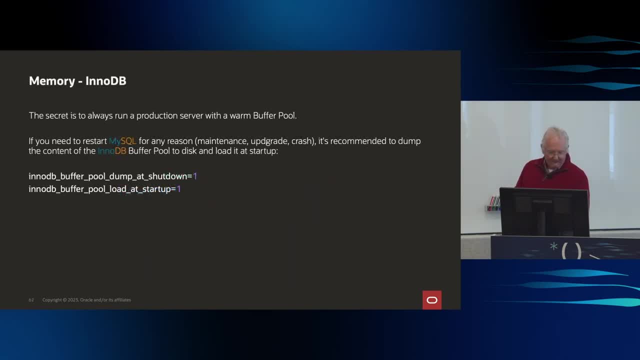 All right. So number seven: memory consumption. So there's a thing called a warm buffer pool, Right? And if you're going to have to stop and start the server and you want to To still be fast when it restarts, then you want to reload the buffer pool. 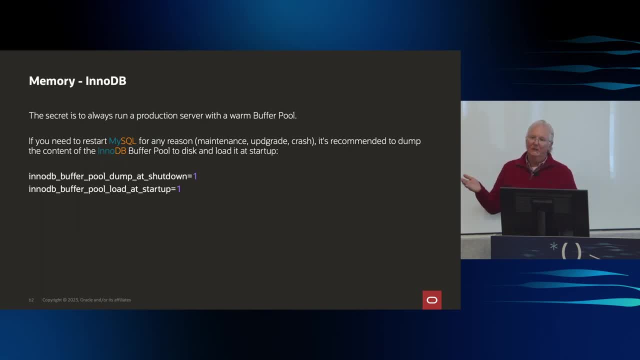 And so you can tell the product to say: I want you to dump that shutdown and I want you to load it at startup Right. And so this is going to. I think the shutdowns will take longer but the startups will have will be performant once it comes up. 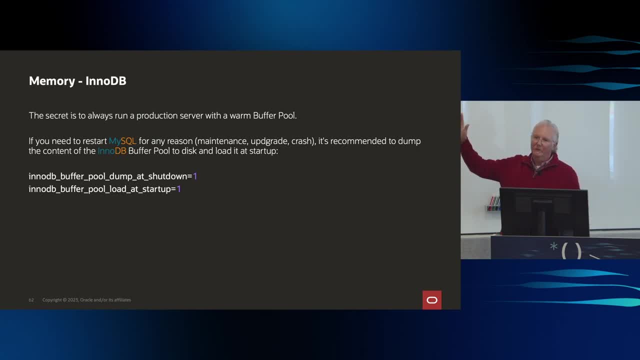 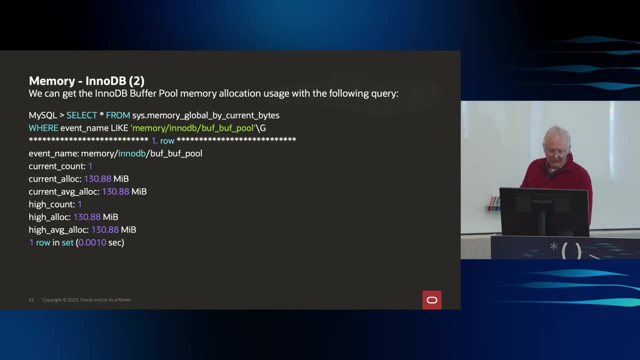 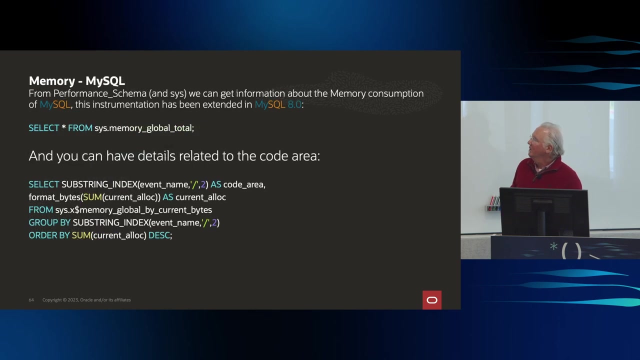 Right, Because now I've got all the pages that were in a buffer pool before I shut down, Right, Right, And the NRDB now, And you can look at the NRDB buffer allocation size and see how many bytes there are And that will sort of give you an idea of how much is going to be written out or read in when you rebalance. 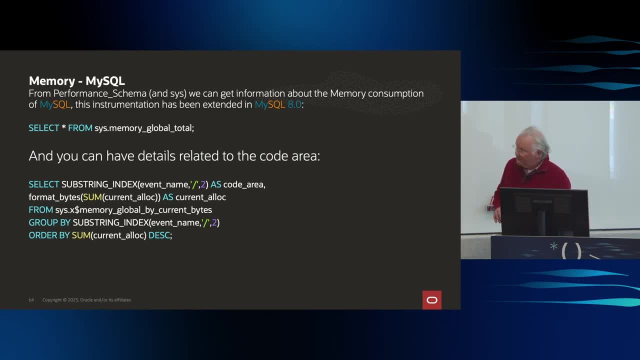 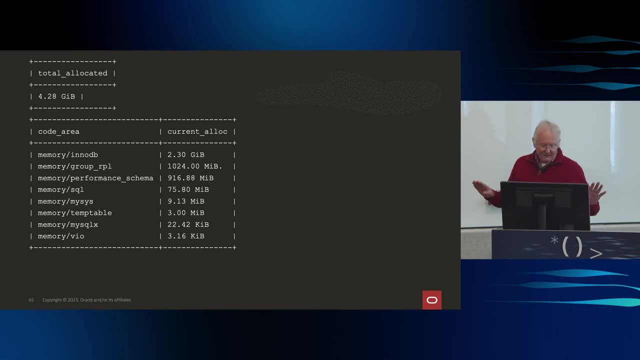 All right, This is about memory consumption And so let's see. So this will give us. OK, I know. So this tells us how much memory is being consumed by the MySQL running instance And it breaks it out by NRDB, by the different components. 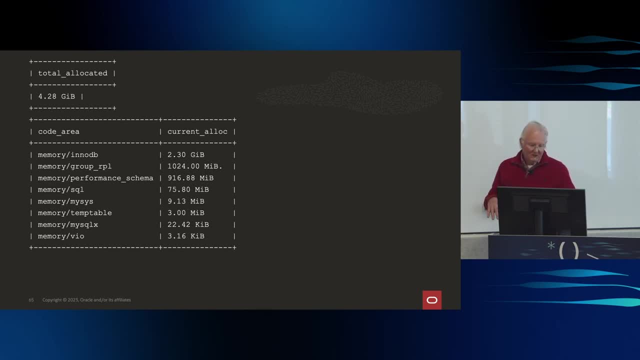 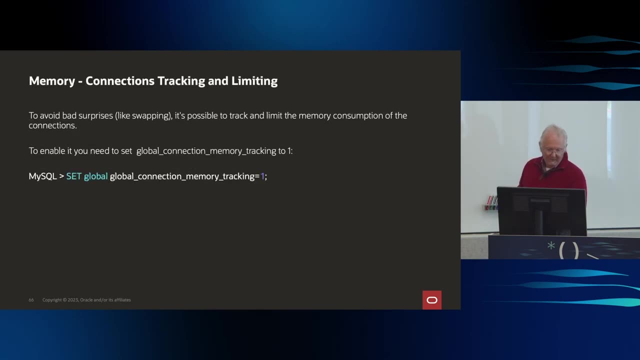 So it's sort of interesting to see what the allocation is And based on that also you know how much RAM you have on the system and things like that. So it's just a good thing to know. Also, another thing that you can limit and that will help performance is that you can track connections. 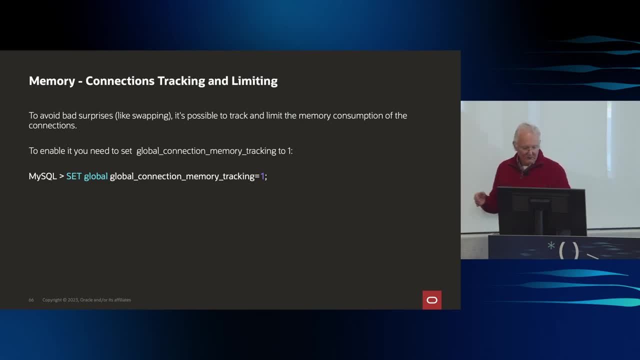 And you can also see how much limit the amount of memory they use. So, one, you can set it to track the connections And two, you can go in and say, hey, I don't want any connection going over this limit. 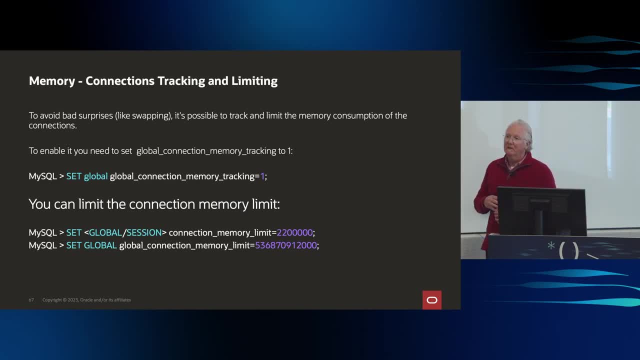 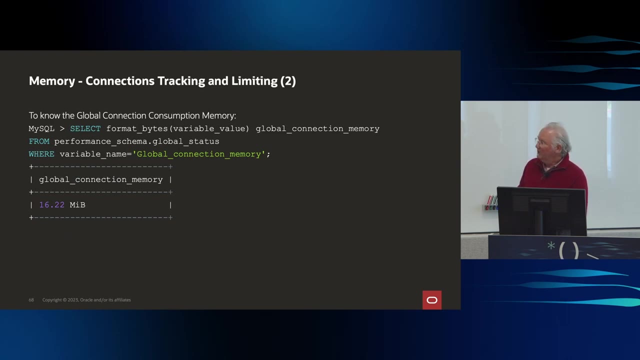 This is probably also a good security type of thing to put in place too, because you want to restrict and not let some denial of service attack or something like that soak up all your memory And so you can look at your global connection memory and use with that particular query. 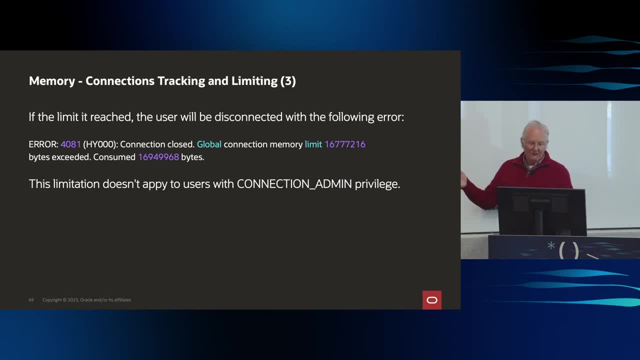 Also, if the somebody does hit the limit, they're going to get an error and it won't be a mystery to you or to them what happened. Right, They ran out of memory for that particular session, for that particular connection. Now it doesn't apply to the. 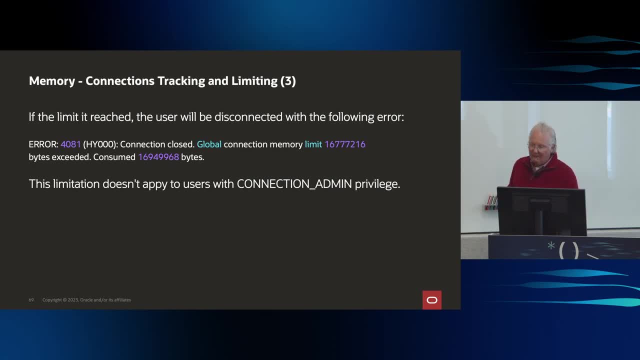 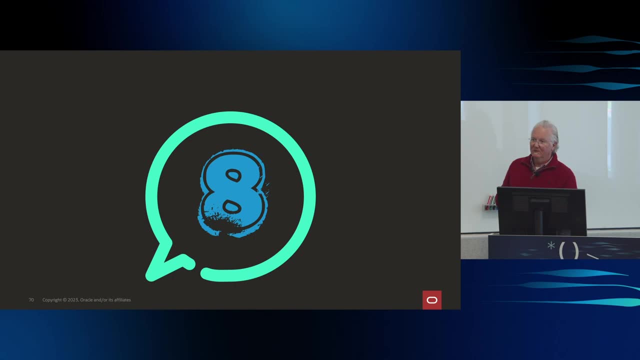 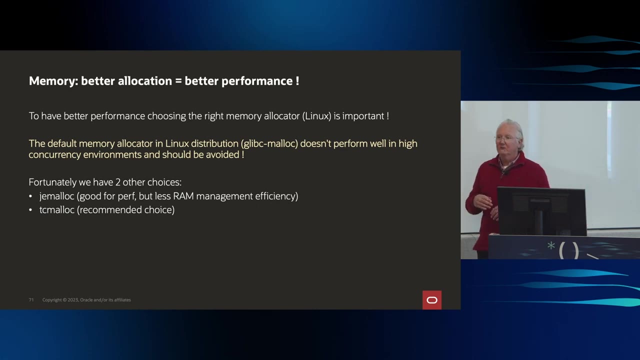 To somebody that's a power user that has the connection, admin Right, The root stuff, All right. Eight, I've got six minutes and two to three to go So On. on Linux, you actually have a choice of what sort of memory allocator you use. 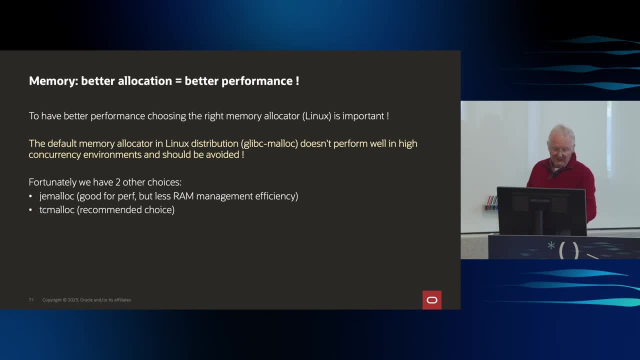 And we have two choices. We have JE Malik, And that's good for performance, But it's not nearly as efficient in RAM as the TC Malik, And that's sort of our recommended choice, And so you can upgrade your Linux to one of these. 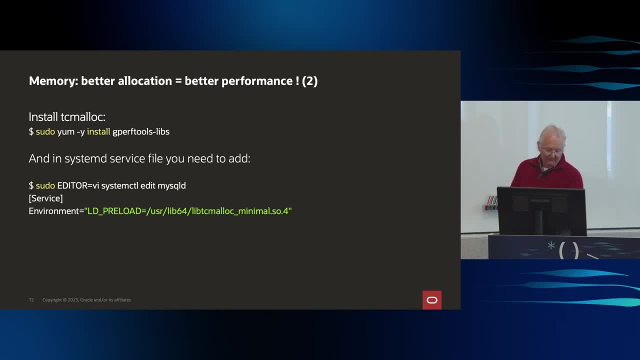 And so you just install TC Malik, for example. this way You edit your system. You really, you know, you really reload, restart the MySQL service, And you start the daemon, And you start the daemon, And you start the daemon. 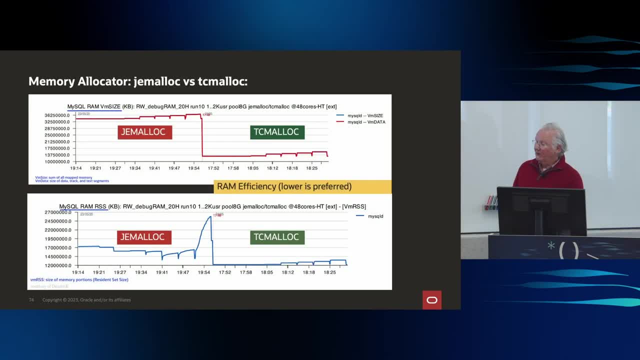 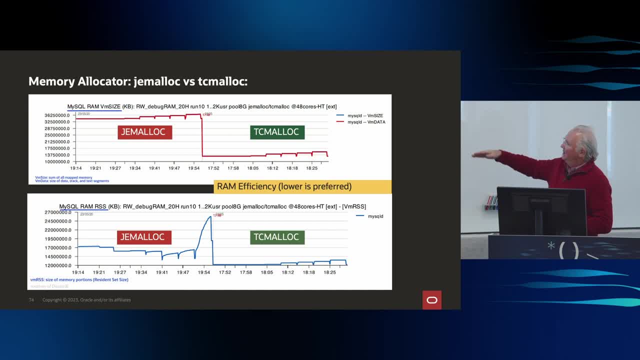 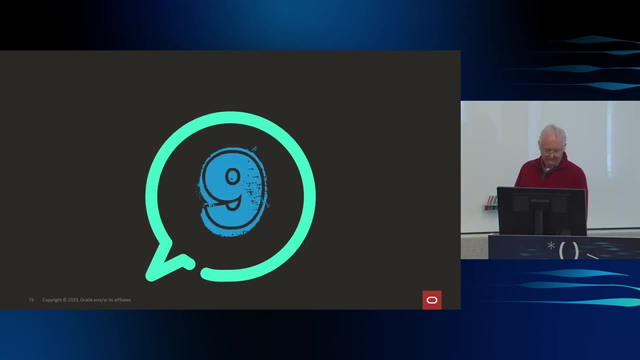 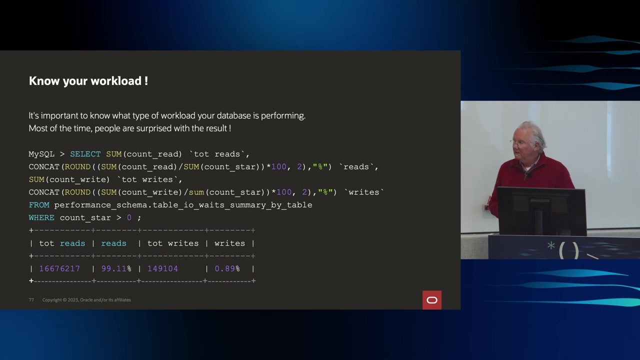 But it's just not as efficient as TC Malik, And so really we recommend you running TC Malik, And this will run faster than just the default one on your system. All right, Number nine: All about queries. So again, it's good to know how many reads, how many writes. 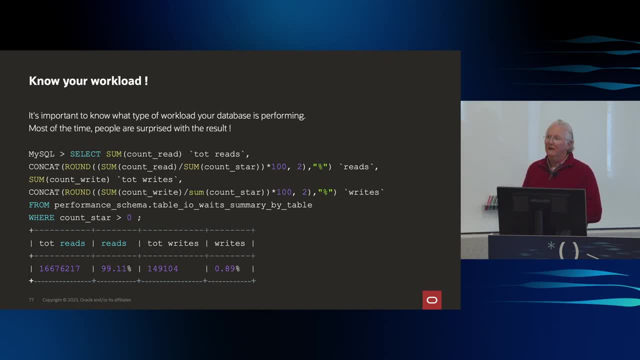 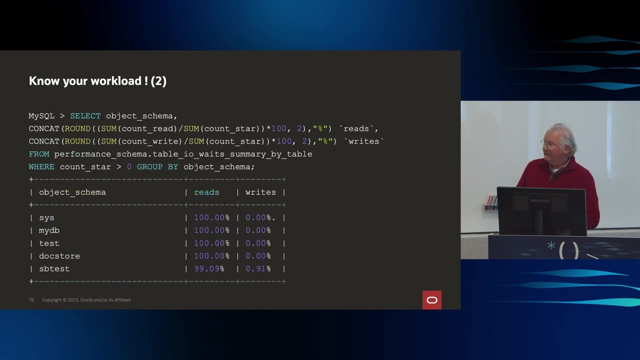 This can tell you also whether you need to do, for example, scale out with the read-only nodes and those sorts of things that we talked about with HA or that the booking guy talked about earlier, And it's also good to know where those are. 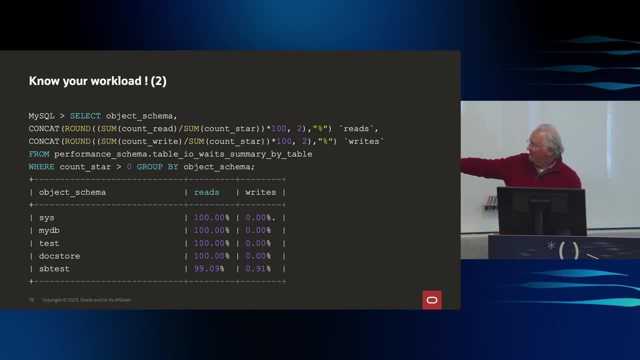 So are they on a particular schema? are they on your document store, whatever test? So this is a way you can tell where these are happening and on what schemas. It may be that you decide that you need to maybe move one of the schemas to a different. 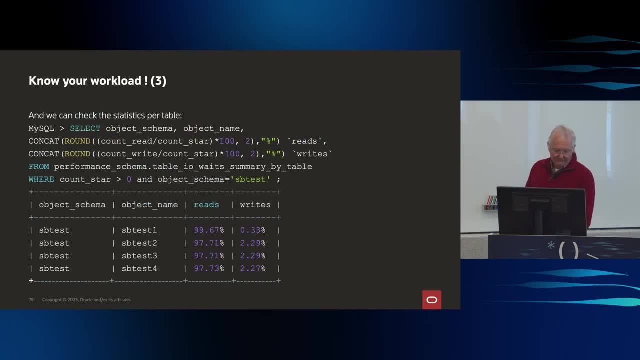 instance, or something like that. So that's how you can check that out, And we can even go all the way down to a per table basis. We can see what each table is doing, how many reads and writes are going on in each table. 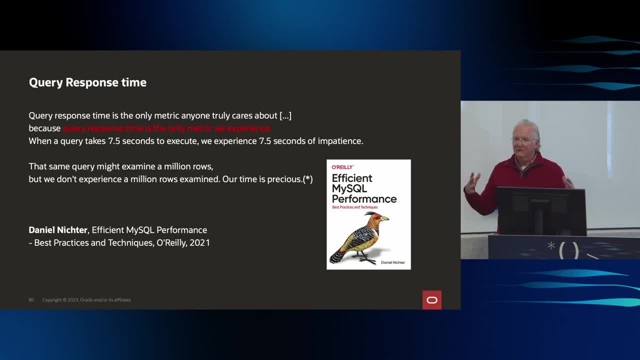 Okay, And these are all sorts of things that we can use to think through what we need to do to have a good query response time and things like that, And this happens to be a book that Laphret likes to recommend on performance tuning that. 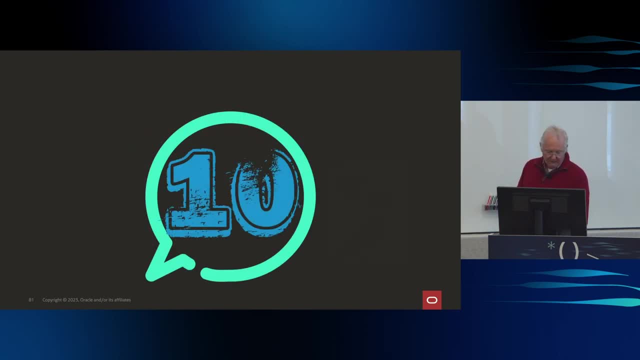 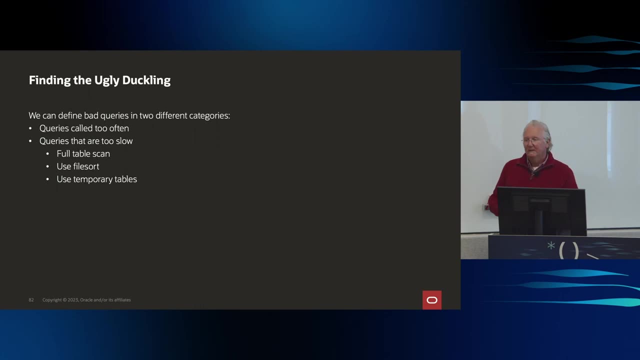 obviously goes into way more detail than what we're talking about today. All right, Number 10. Find the ugly duckling, So at some point you just have to start looking at what to tune, And so Okay, So you know whether it's queries called too often, queries that are too slow doing. 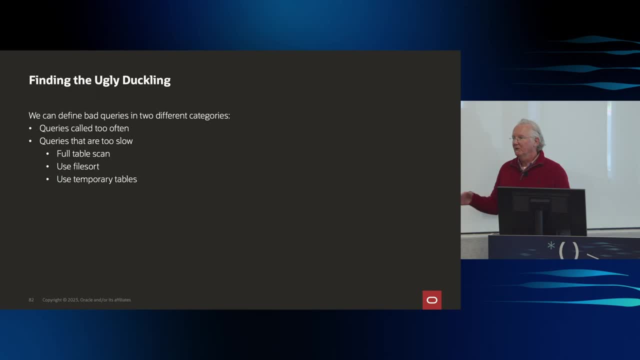 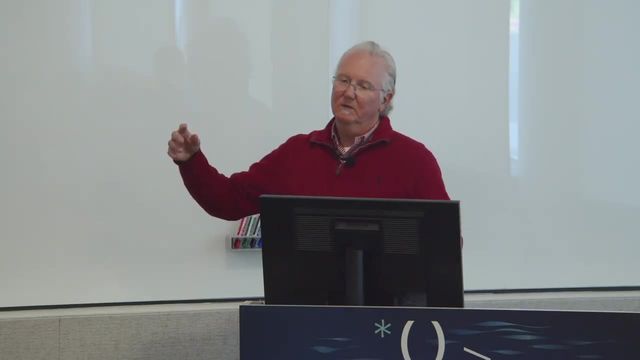 full table scans or file sorts or looking, you know, using a lot of temporary table space. these are all sort of things that will slow you down right And really you want the one that's using up the most saturating, the most usage on your. 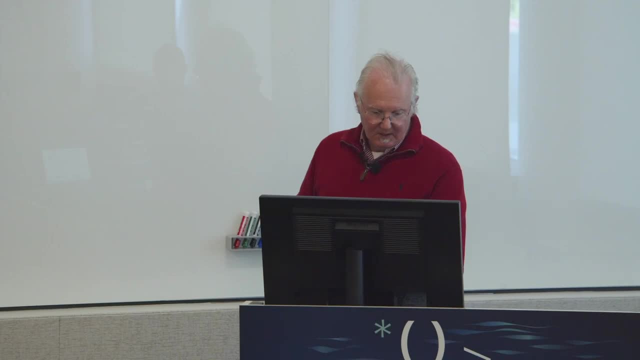 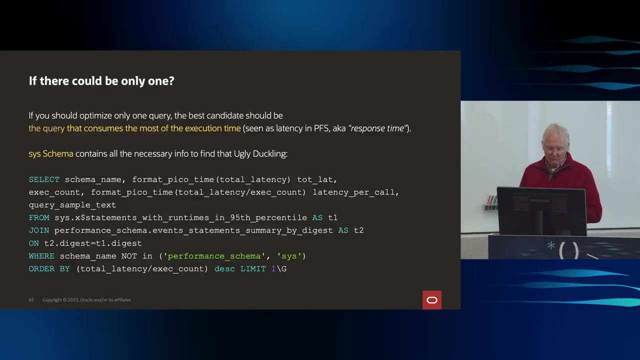 server right, But the easiest ugly duckling to find is the one that consumes the most execution time, Because that's most likely your most problematic one, And so we can query the sys schema with this particular call, And it's going to pop out. 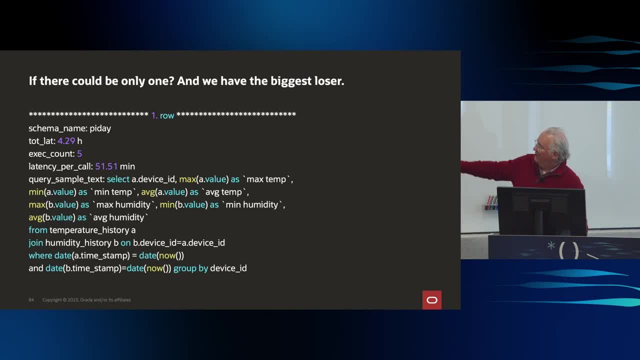 And it's going to tell me what that query is. that is so bad, right, And so this happens to be the one that it found. And this thing is, you know, 51 minutes, right? So it's horrible latency, right. 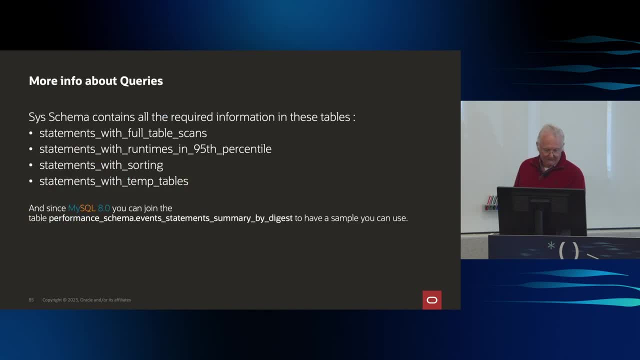 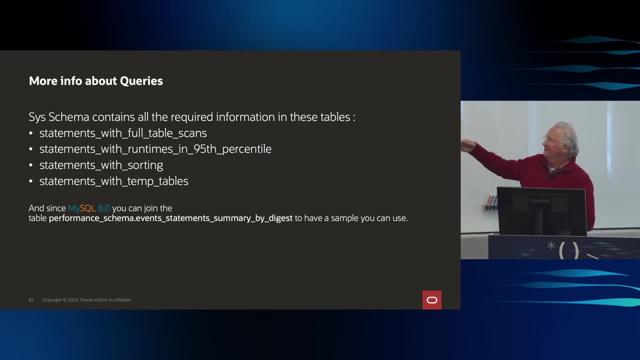 This is another way to find ugly ducklings: Statements with sorting- There's a sys schema view on that- Or statements with temp tables. So again, all these things are ugly ducklings. All these sys views are there. They're there to just make them present to you, so it's easy to find. 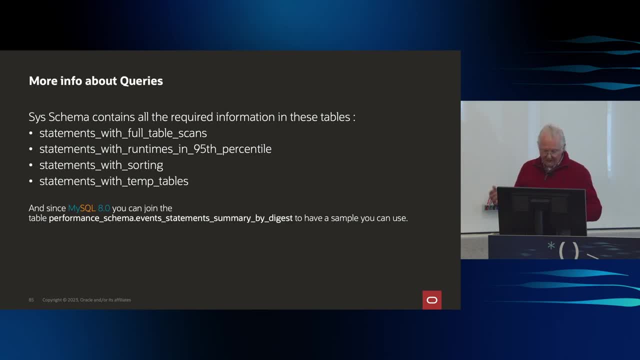 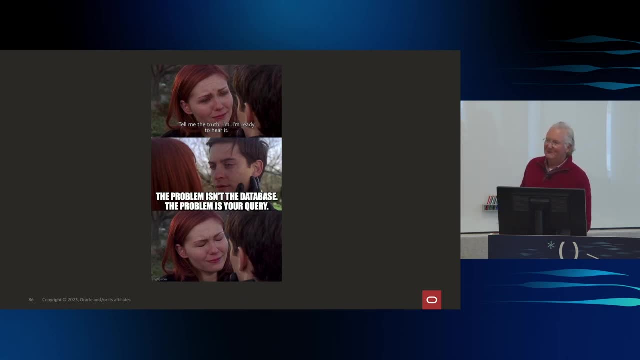 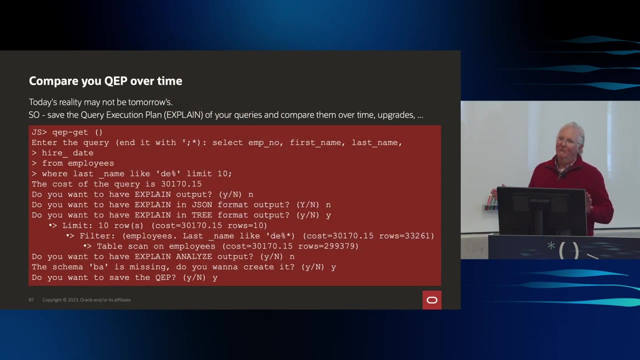 These are easy things to query And you can go in and try to figure out what to do. So the problem isn't with the database, The problem is your query. So, and the point of that is that you need to watch your queries-